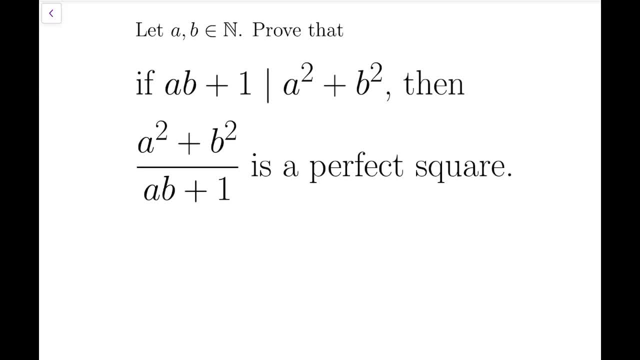 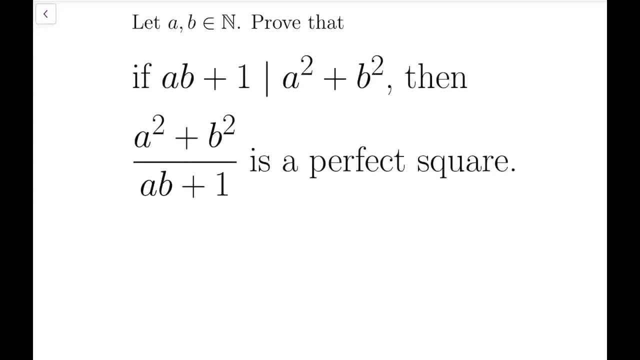 So in this video, I'm going to share with you a very elegant, intelligent solution produced by Mr Immanuel Atanasov from Bulgaria. The trick used in this solution is later named as Vieta Jumping- Starting off with a solution, we can rewrite the given expression into a quadratic equation. 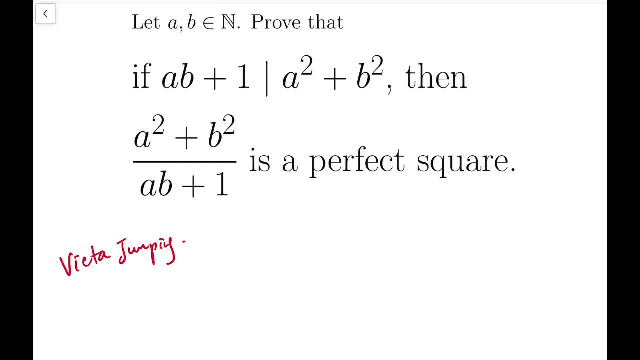 and with the help of the Vieta's formula, which involves sum and product of roots of polynomial equations, we can generate, or in other words jump to another solution which is smaller than the one we started with. But iterating, something will go wrong. 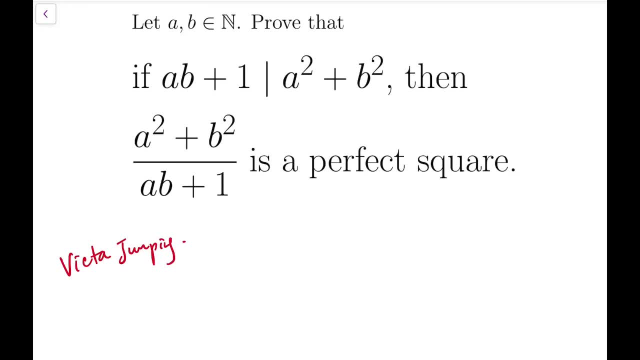 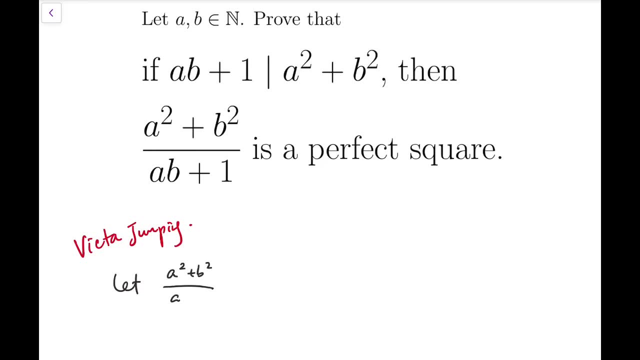 This is actually very similar to the infinite descent trick, so let's see how it works. So I'm going to start off by letting a squared plus b squared over a plus one equals k, which is some integer or, to be more precise, a natural number. 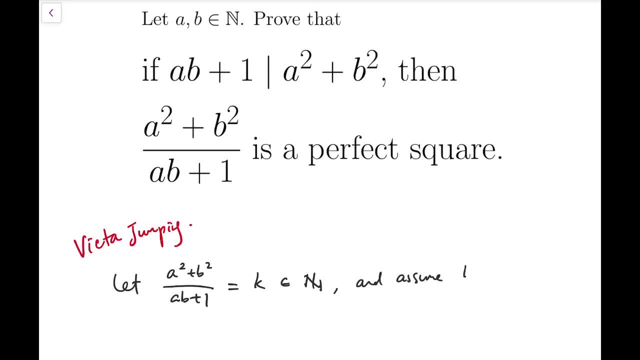 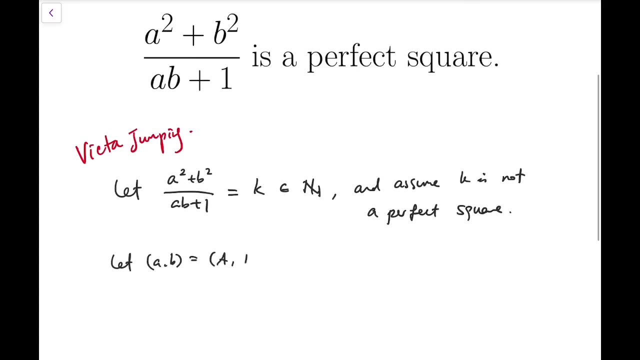 that is, from the given condition, And of course we assume that it's not a perfect squared. Starting with a proof by contradiction, Now let one of the solutions to be big A, big B, be a solution to the above equation such that 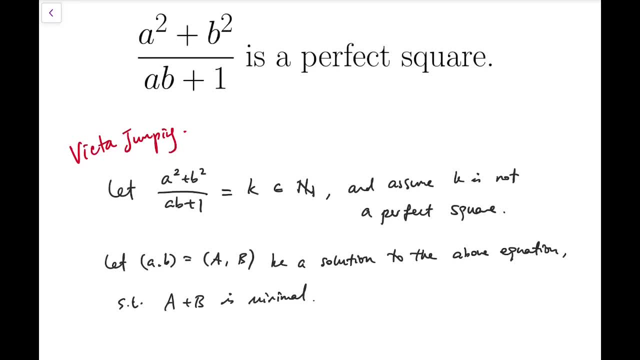 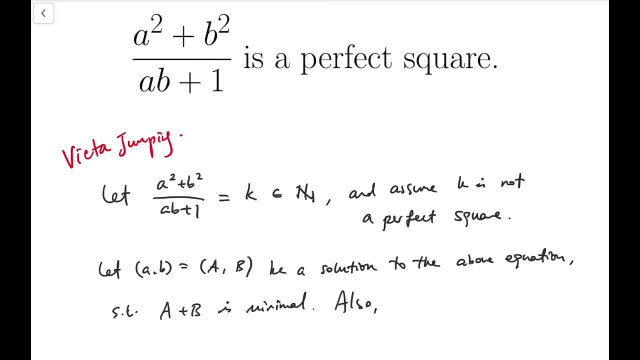 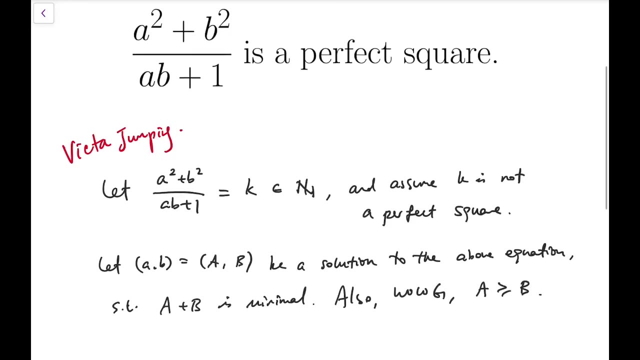 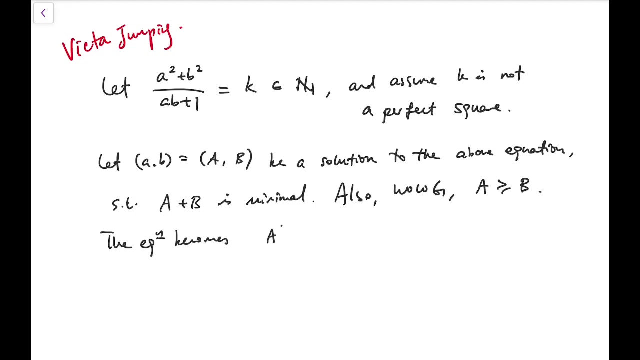 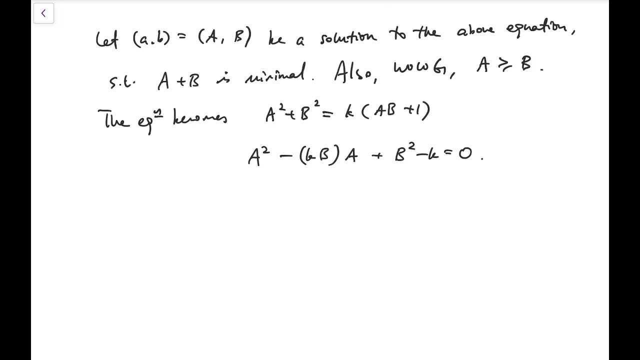 a plus b is minimum. Also, by symmetry of the above equation I can say, with the loss of generality, a is larger than or equal to b, So that equation becomes: a squared plus b squared equals k times a, b plus one, And so a squared minus k. 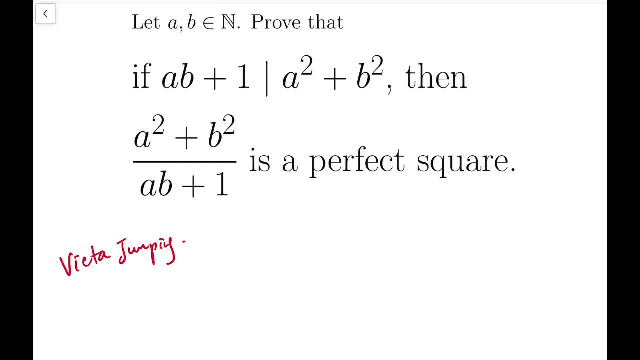 and with the help of the Vieta's formula, which involves sum and product of roots of polynomial equations, we can generate, or in other words jump to another solution which is smaller than the one we started with. But iterating, something will go wrong. 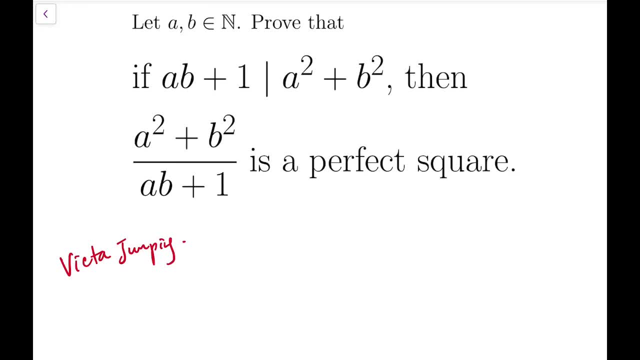 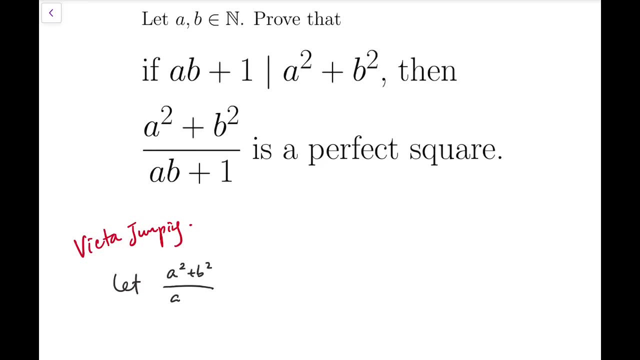 This is actually very similar to the infinite descent trick, so let's see how it works. So I'm going to start off by letting a squared plus b squared over a plus one equals k, which is some integer or, to be more precise, a natural number. 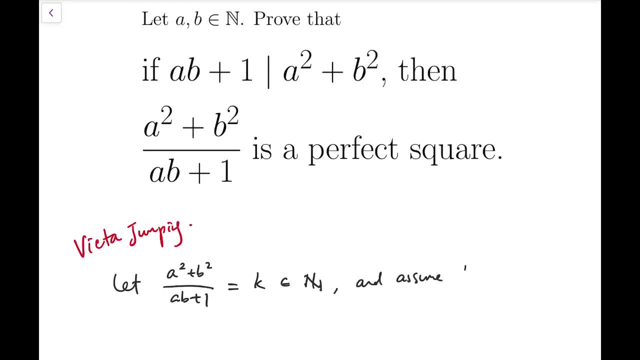 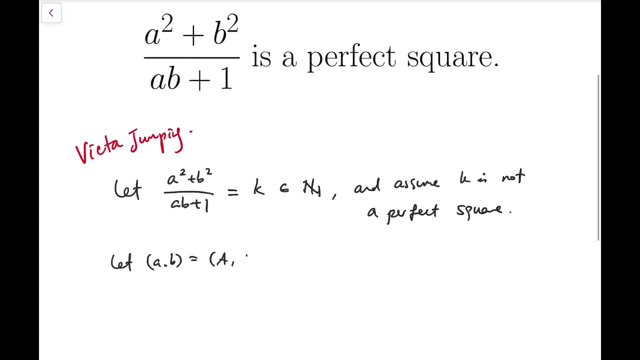 that is, from the given condition, And of course we assume that it's not a perfect squared. Starting with a proof by contradiction, Now let one of the solutions to be big A, big B, be a solution to the above equation such that 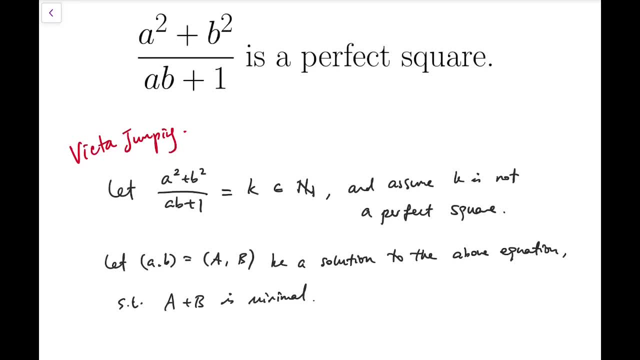 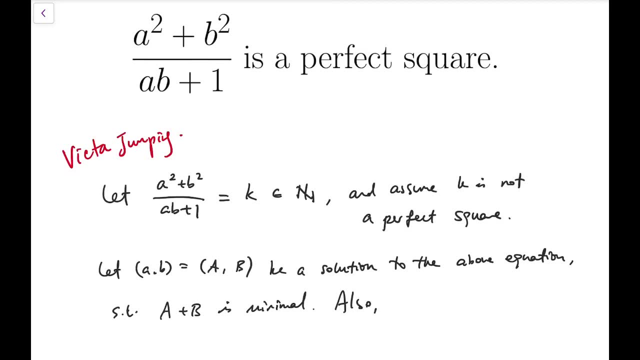 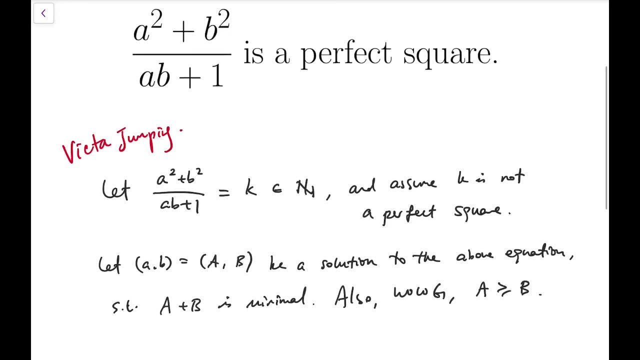 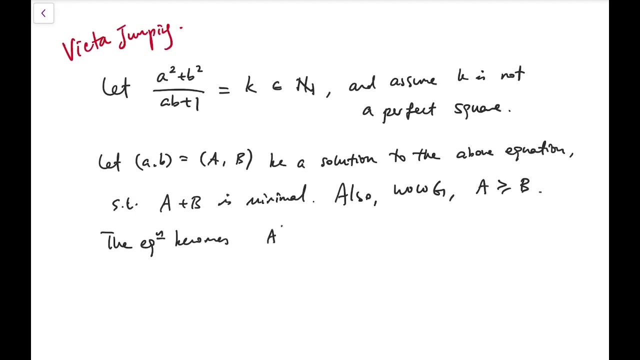 a plus b is minimum. Also, by symmetry of the above equation I can say, with the loss of generality, a is larger than or equal to b, So that equation becomes: a squared plus b squared equals k times a, b plus one. And so a squared minus k, b times a plus b squared minus k, equals zero. 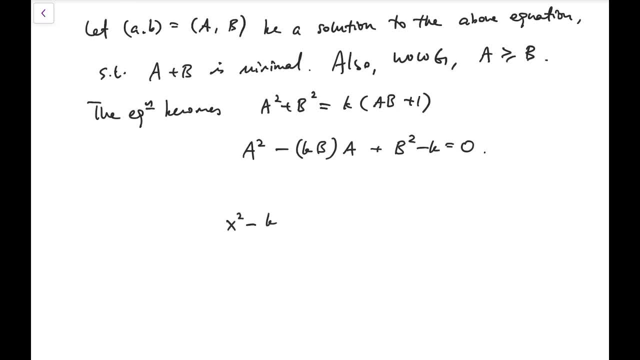 That means this big A is the root to the equation. x squared minus k, b times x plus b squared minus k equals zero, And for this qualitative equation surely there must be a second root. So I'm going to let a and a1 be the roots to this equation. 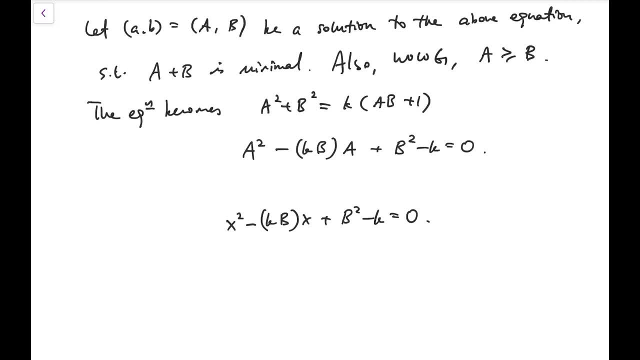 b times a plus b squared minus k, equals zero. Now that means a. this big A is the root of the equation. x squared minus k, b times x plus b squared minus k equals zero. And for this fingertip equation surely there must be a second root. So I am going to let x squared equal to k for the argument. 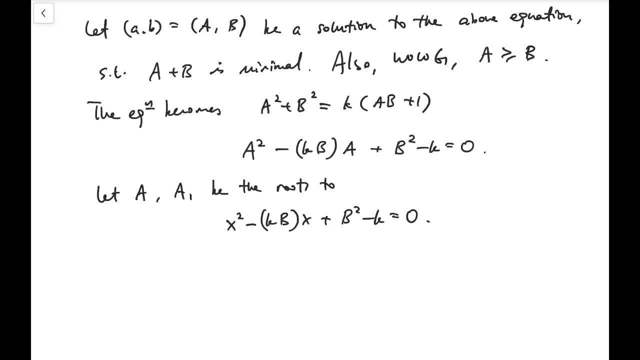 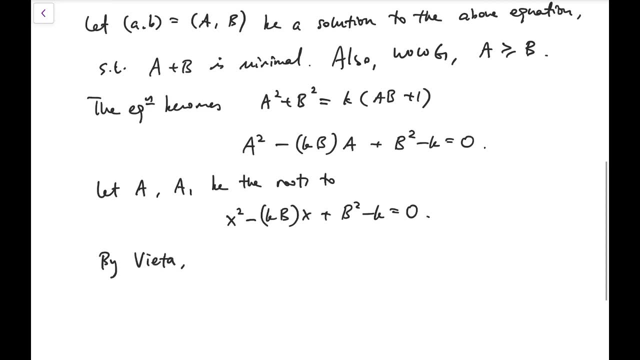 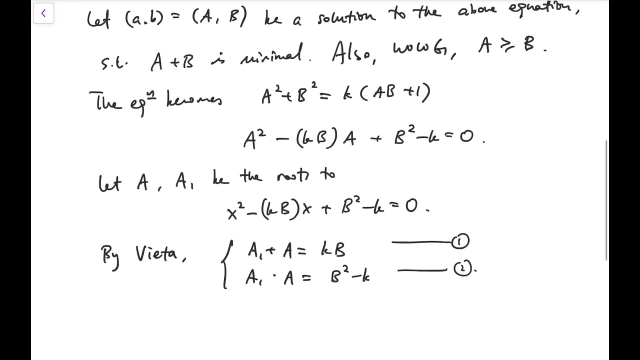 Let A and A1 be the roots to this equation. And now I can bring in the Viettas formula. The sum of roots should be KB and the product is B squared minus K. Okay, the aim of using the Viettas formula is to show that this A1, the second root, 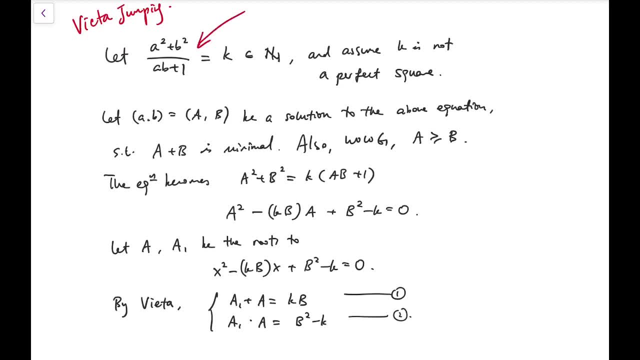 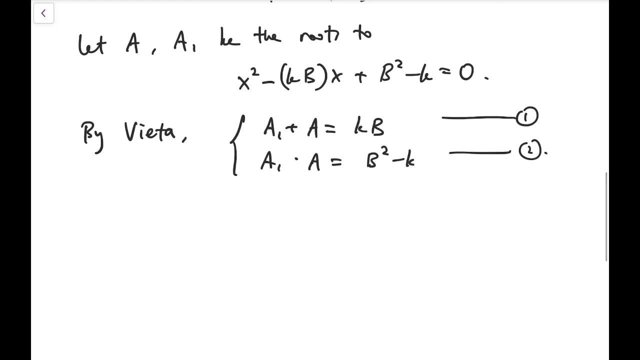 is not just simply the root of this project equation, but also a valid solution to the original expression, Which is that, in other words, I'm going to show that this big A1 is a positive integer. So, from the first equation, big A1 is KB minus A. 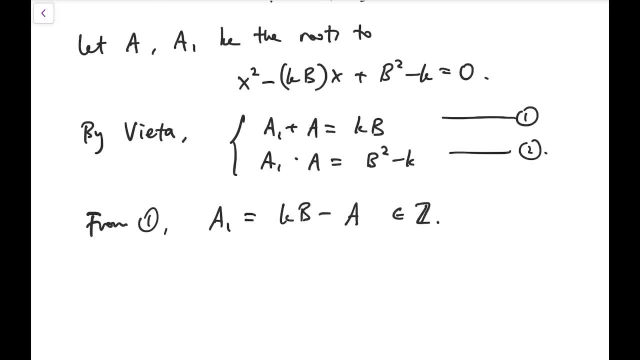 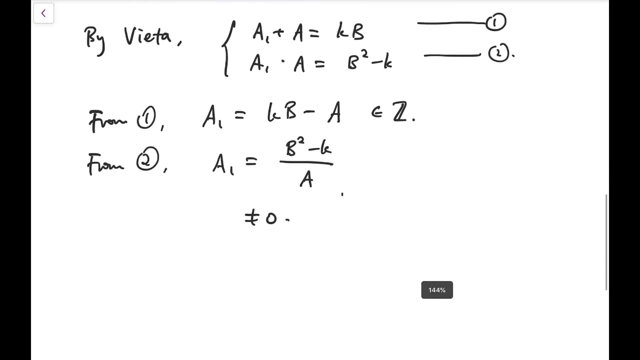 And because K, B and A are all integers, we know that big A1 is an integer From the second equation. A1 equals B squared minus K Over big A. And because K is not a perfect square, surely this is not zero. 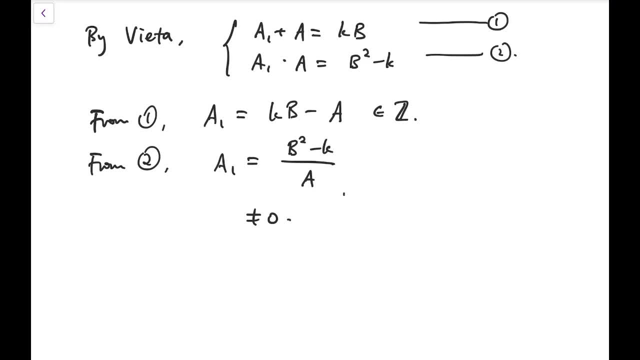 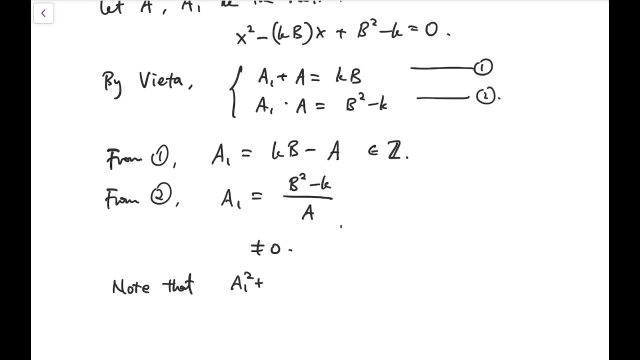 So we've shown that it's an integer and to show that it's positive, we need to show that it's not zero and also that it's not negative, Noting that the fact that big A1 is a root tells us that this big A1 is a positive integer and that this big A1 is a positive integer. 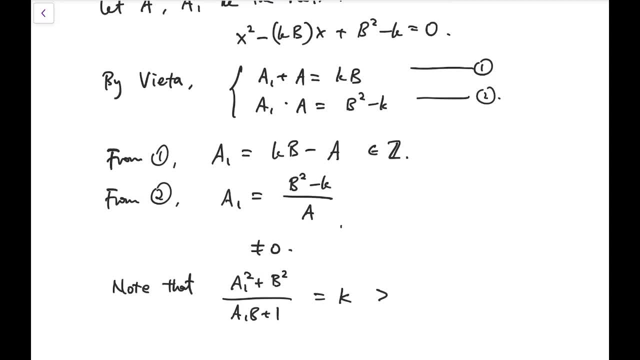 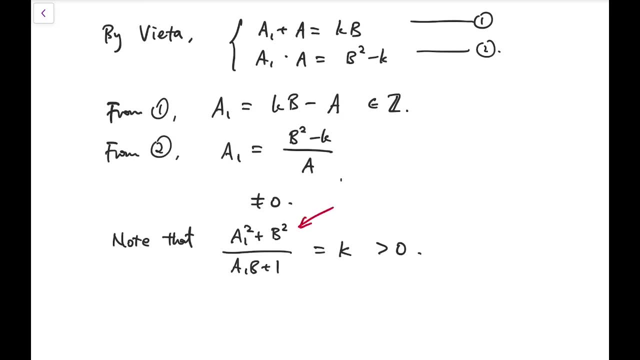 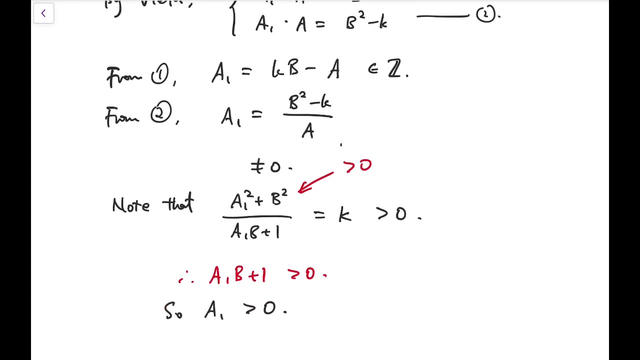 This expression equals K, and this K is positive, Together with the fact that A1 squared plus B squared is also positive. this part- A1B plus 1, should also be positive, And from this we can already tell that big A1,. 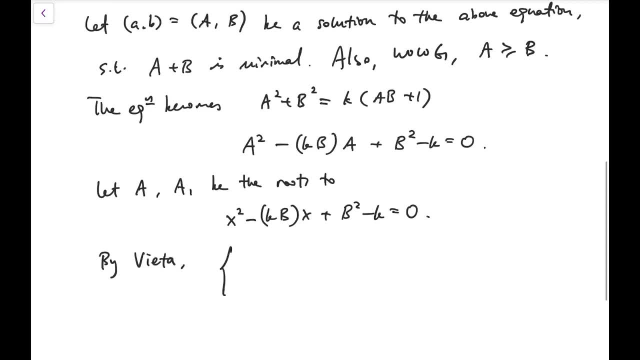 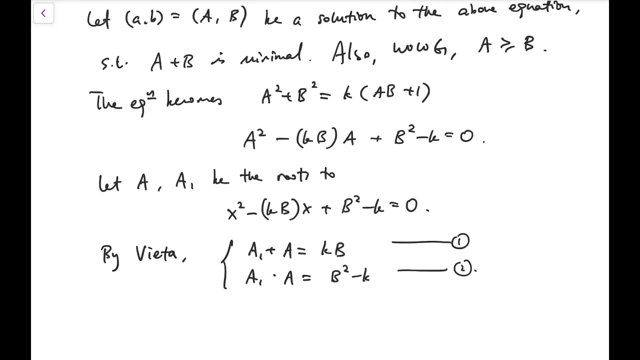 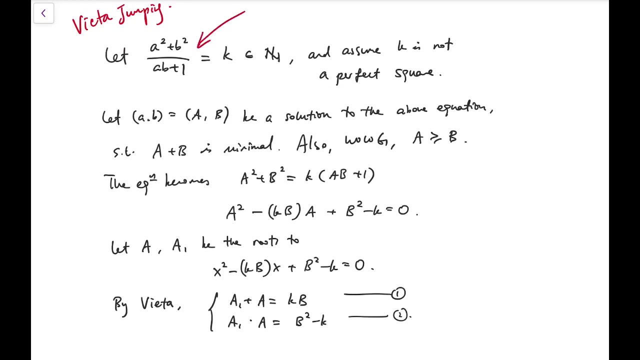 And now I can bring in the Viettas formula. The sum of roots should be kb and the product is b squared minus k. Okay, the aim of using the Viettas formula is to show that this a1, the second root, is not just simply the root of this project equation, but also a valid solution to the original expression. 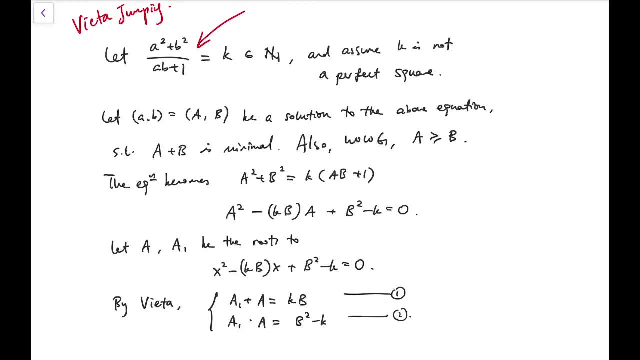 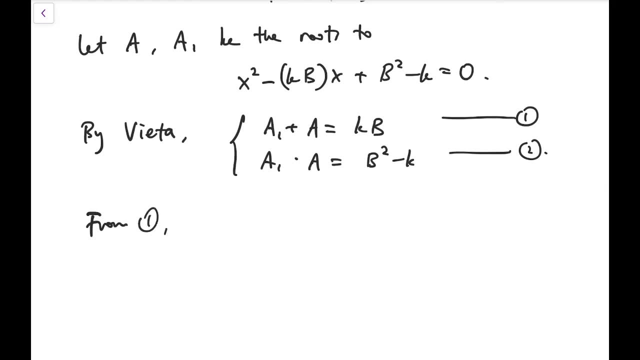 Which is that, in other words, I'm going to show that this big a1 is a positive integer. So, from the first equation, big a1 is kb minus a, And because k, b and a are all integers, we know that big a1 is an integer. 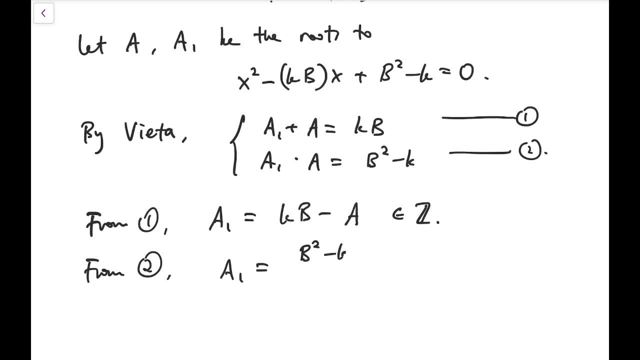 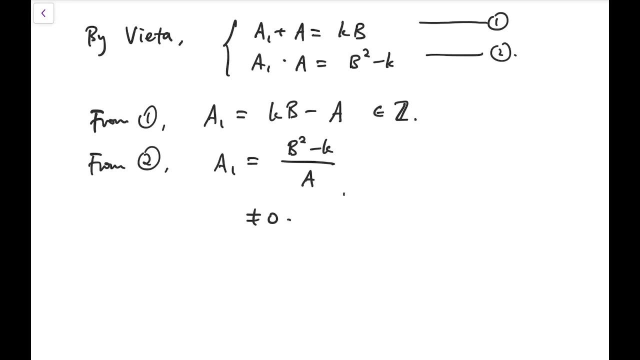 From the second equation: a1 equals b squared minus k, And because k is not a perfect square, surely this is not zero. So we've shown that it's an integer and to show that it's positive, we need to show that it's not zero and also that it's not negative. 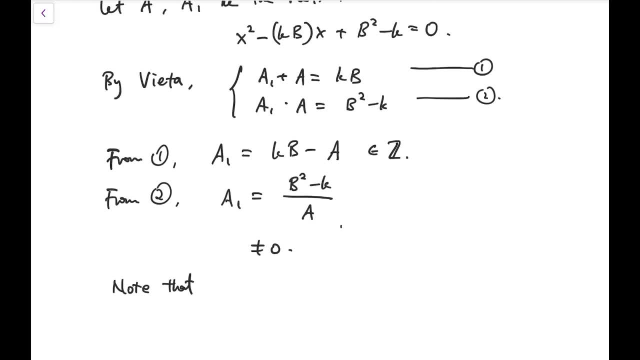 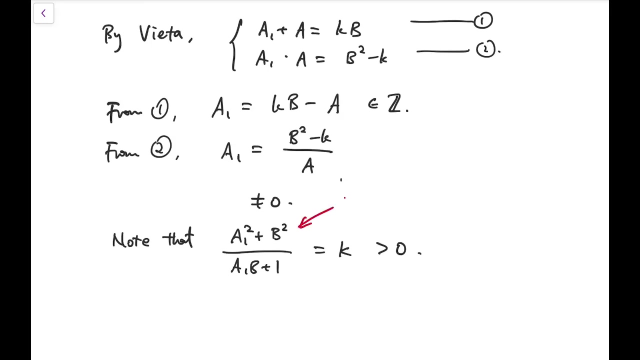 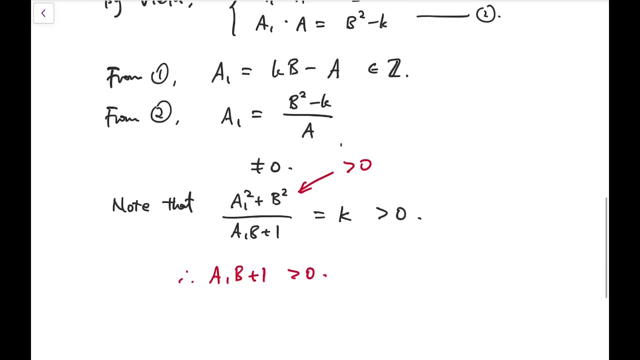 Noting that the fact that big a1 is a root tells us this expression equals k and this k is positive, Together with the fact that a1 squared plus b squared is also positive. this part- a1, b plus 1, should also be positive. 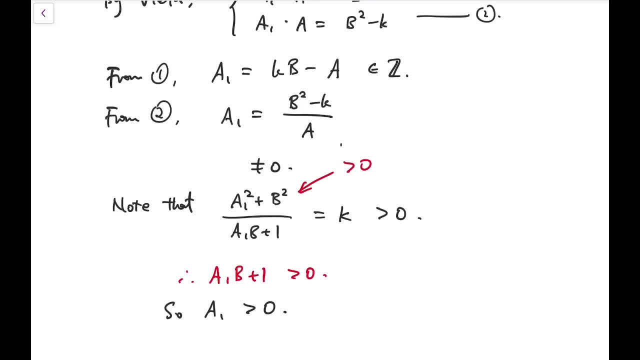 And from this we can already tell that big a1 is a positive integer. And from this we can already tell that big a1 is a positive integer. And from this we can already tell that big a1 is a positive integer. 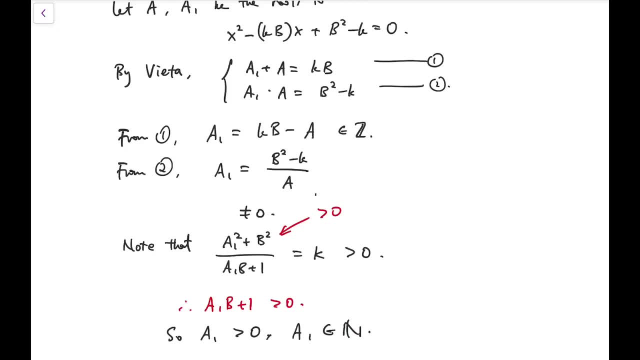 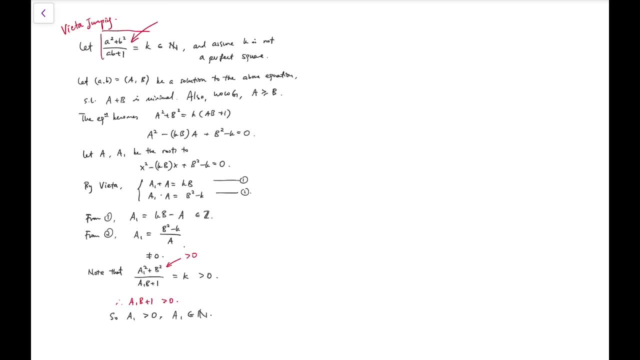 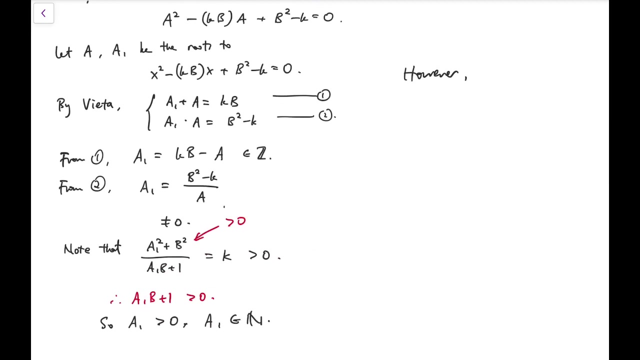 So because it's positive as an integer. so, therefore, a1 is a natural number, which means it's a valid solution to the above, to the starting expression. this one, However, this one, this big a1, is in fact a smaller solution than the one that we start off with. 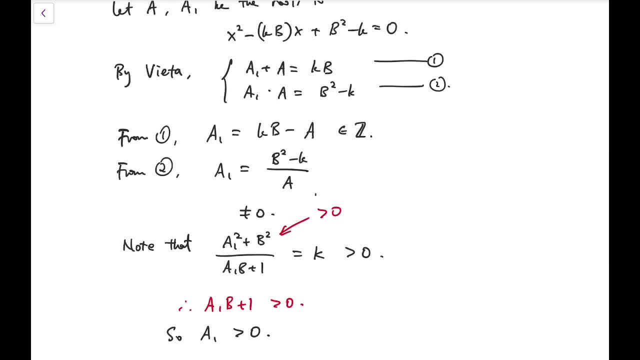 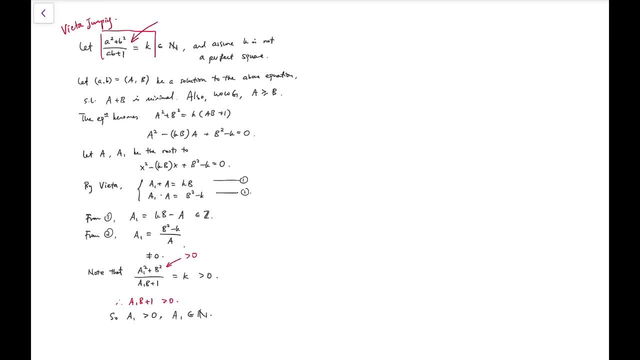 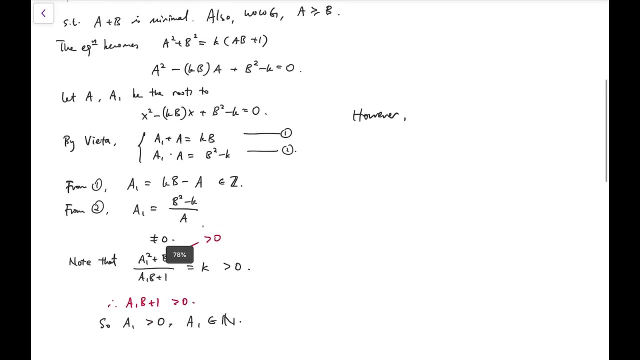 A1 is positive, So because it's positive as an integer. so therefore, A1 is a natural number, which means it's a valid solution to the above, to the starting expression. this one, However, this one, this big A1,. 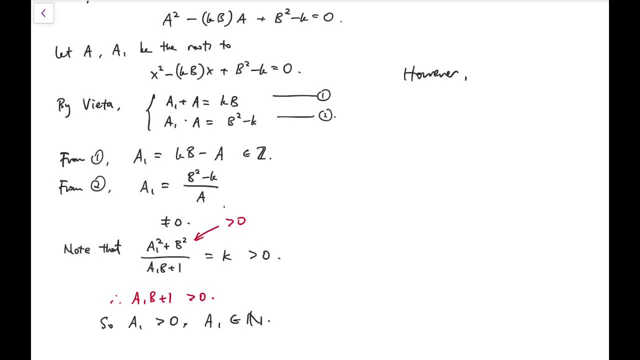 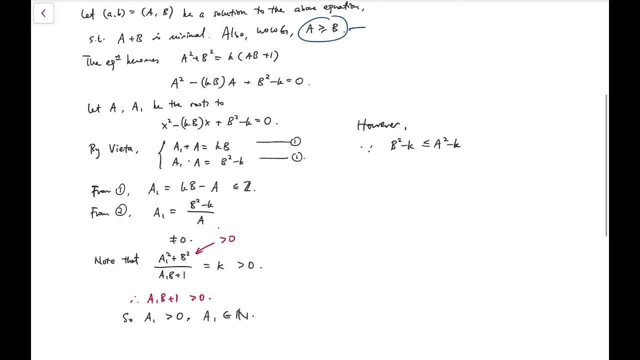 is in fact a smaller solution than the one that we start off with. This is because B squared minus K is less than or equal to A squared minus K by the assumption that we have made with the loss generality, And this is clearly smaller than A squared. 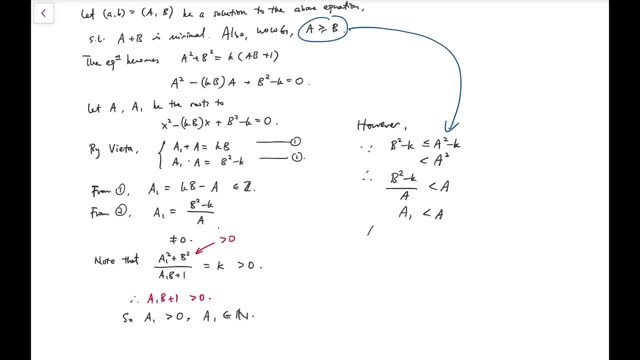 So B squared minus K over a is more than a, which means a1 is more than a. So a1 plus a1 and b is another solution, but the sum of the two numbers is more than a plus b, which contradicts its minimality. 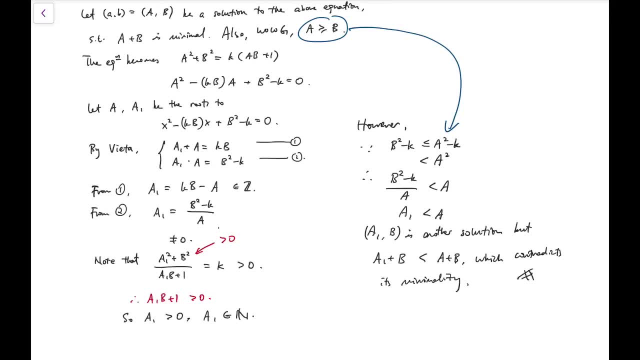 And this contradiction only arises because we've assumed that k cannot be a perfect square. So therefore, a squared plus b squared over a, b plus 1 must be a perfect square. So yeah, we are done. I hope you enjoyed the video. Feel free to suggest. 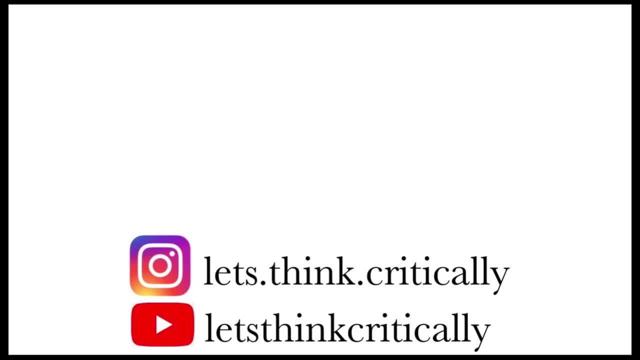 any alternative questions. If you like my videos, make sure to subscribe to my channel right now. Thank you for your support. See you next time.